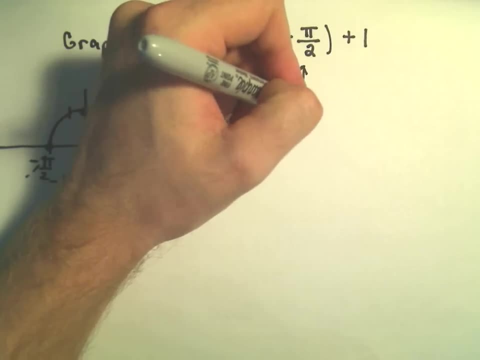 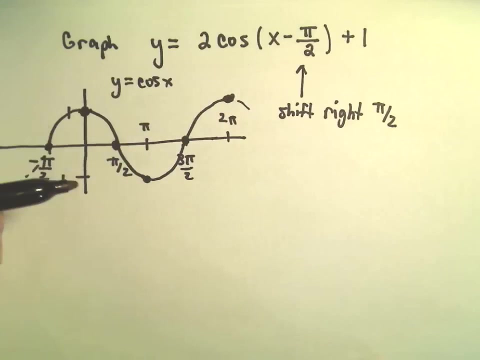 And since we see negative pi over 2, again, this means we're going to shift the graph of cosine to the right by pi over 2 units. I'm going to do another thing at the same time as well, And all the 2 is going to be negative. 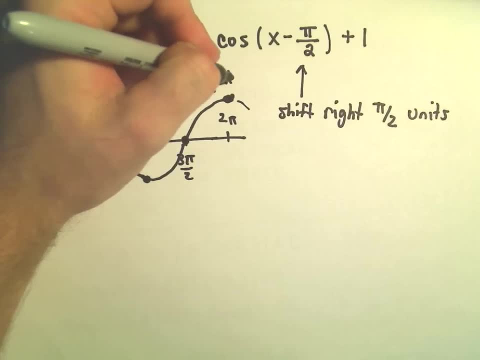 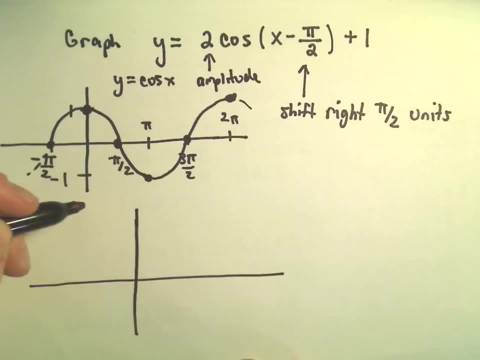 So what I'm going to do is just going to change the amplitude. So, instead of going up to positive 1 and negative 1, we'll now go up to positive 2 and to negative 2.. So let's see, Let's try to shift everything. 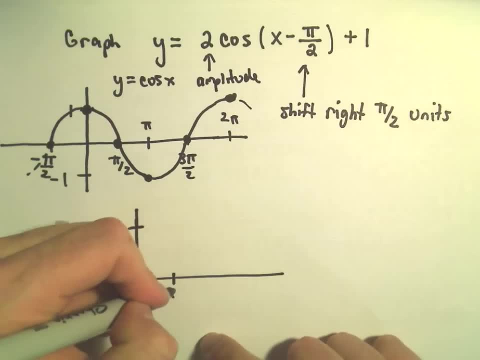 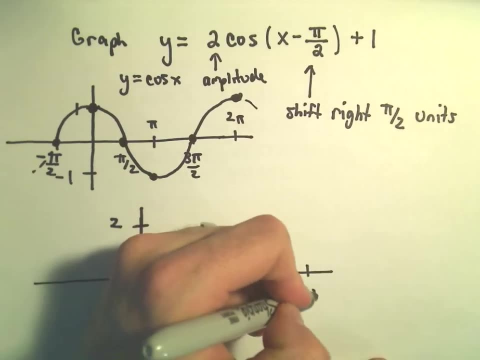 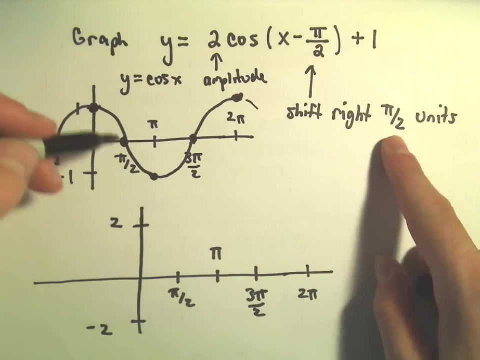 So there's positive, 2. There's negative, 2. Pi over 2, pi 3, pi over 2, and then 2 pi. Okay, at 0, we were originally at 1.. So if we shift that over pi over 2 units again, then we would have been at pi over 2, comma 1.. 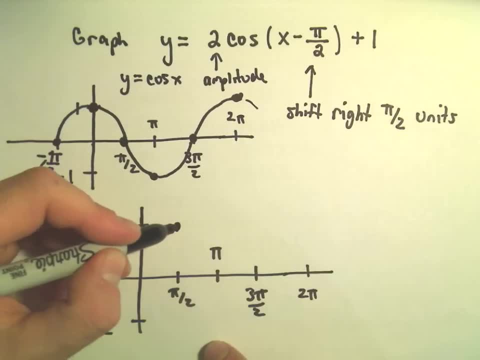 But again, because of this amplitude it'll now be up here at pi over 2, comma 2.. The original point that was at pi over 2, 0, if that gets shifted over pi over 2 units we would now be sitting at pi. 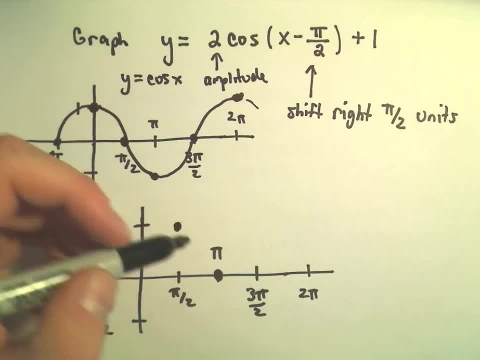 So we'll still be getting 0 out there At 3 pi over 2,. let's see So, if we take the value that was at pi, we add positive At negative 1, or, excuse me, negative 1.. 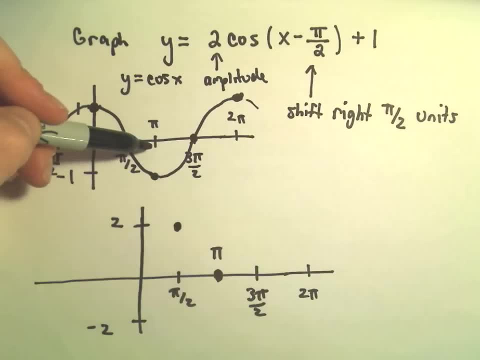 At pi we add negative 1.. So when we change the amplitude that'll go from pi down to negative 2.. But again we're just moving that point over: pi over 2 units. So at 3 pi over 2, we'll be down here at negative 2.. 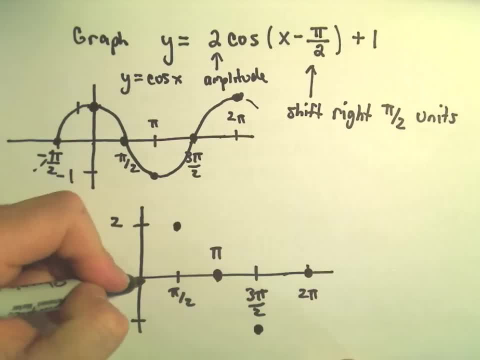 And then we'll be back at 0,, et cetera. All right, so I think we've got our kind of rough graph here. Let's see: So, at negative pi over 2, we would be down here at negative 2.. 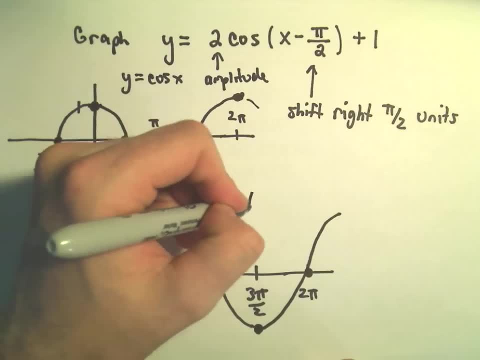 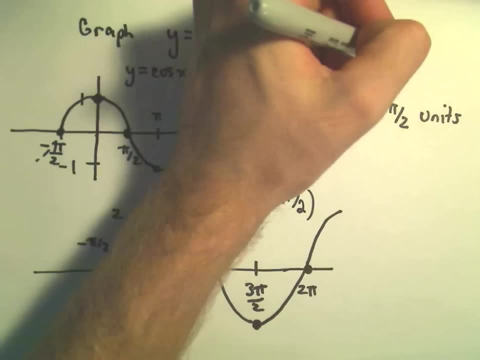 So now we've got a rough graph of 2 cosine of x minus pi over 2.. And, last but not least, all we have to do, remember this: plus 1 is going to be a vertical shift And the plus 1 is just going to shift the graph. 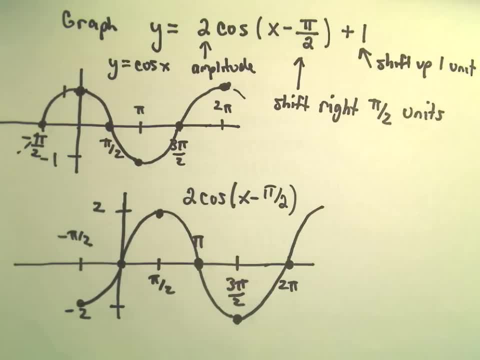 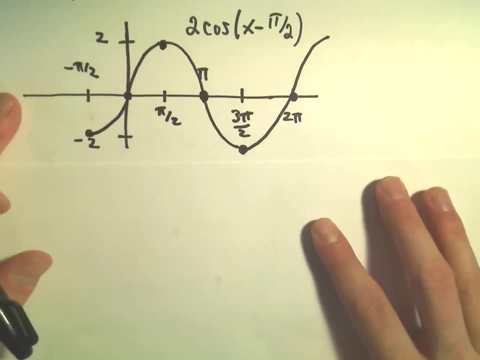 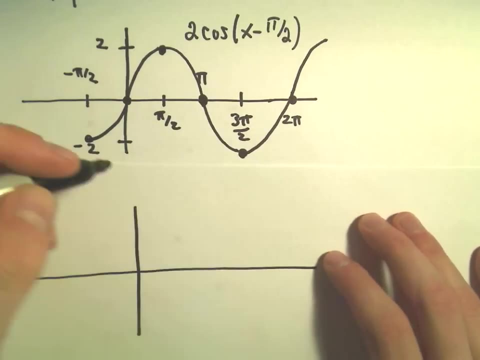 It'll shift the graph simply up one unit. So grab another piece of paper here. So now I'm just going to simply take this, Take this original graph that we came up with and shift it up just one unit. Okay, so instead of being at 0, 0, we'll now be at 0, comma 1.. 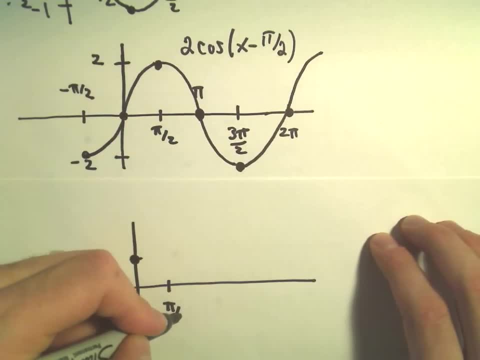 Instead of being at pi over 2, comma 2, we'll now be up here at pi over 2, comma 3.. And again, instead of being at pi 0, we'll now be at pi comma 1.. 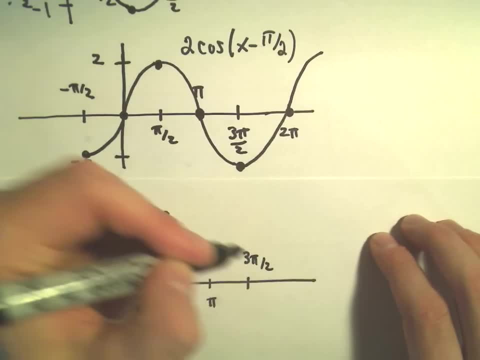 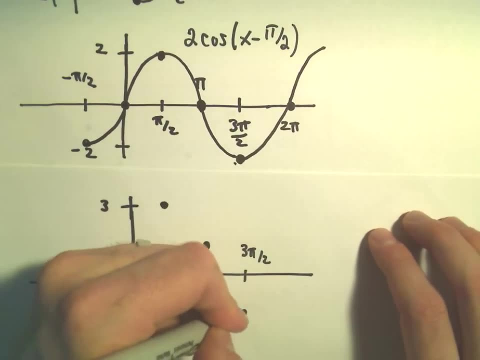 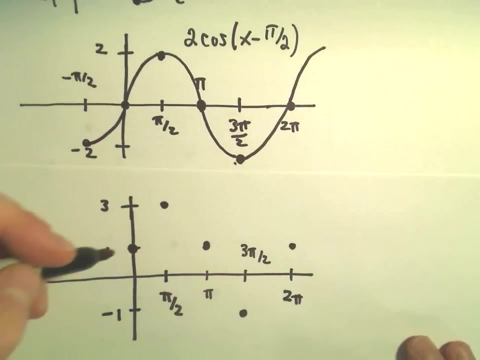 At 3 pi over 2,, instead of being at the y-value of negative 2, we'll now be at the y-value of negative 1.. And then, when we're back at 2 pi again, instead of being at 0,, since we've added 1, we'll now be one unit higher. 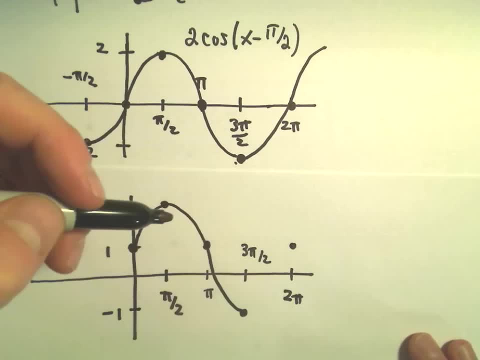 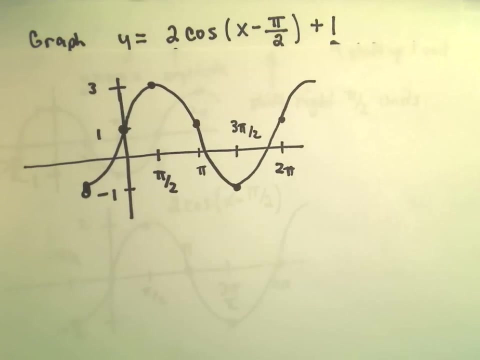 So now we've got that same graph that we had before. It's just that things have been shifted up one unit. So that's pretty much all there is to it. But you know, this is kind of how you know. if you told me to graph this original thing, this would exactly. you know, this is exactly my thought process. 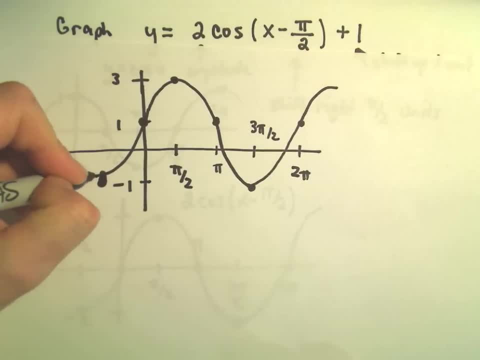 I kind of do it just a little step at a time and I kind of make them stop here Again. they definitely keep going, But this is how I do it. I kind of shift it to the right pi over 2 units. 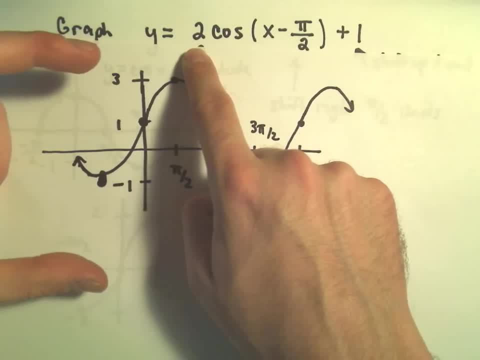 I think about this amplitude, how it's kind of stretching the graph out, And then I just take that whole thing and move it up one unit because of the plus 1..